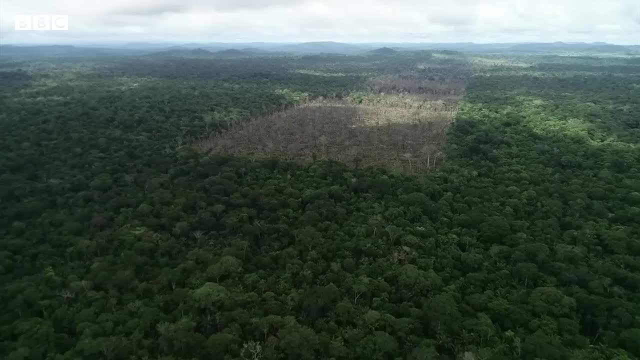 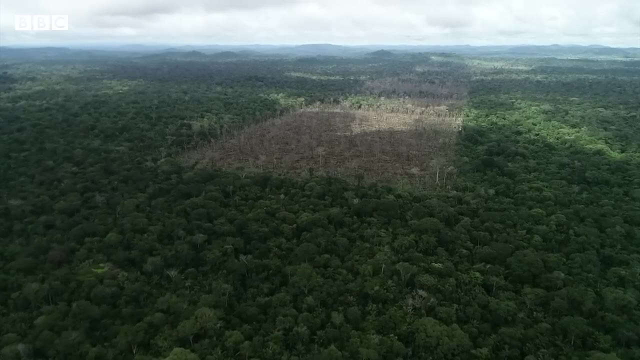 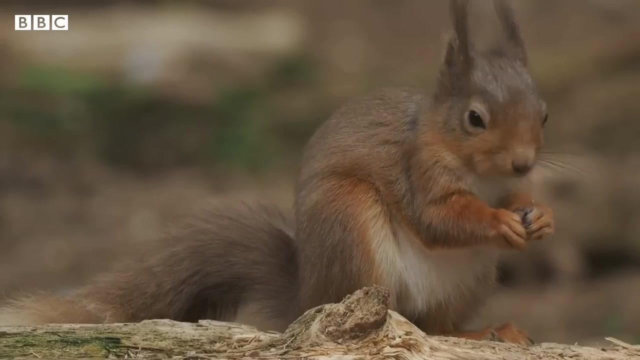 And the species who rely on them to sustain life. Wildlife population sizes here have fallen by 94% over the past half century, according to the report. Other areas such as North America, Asia and Europe have seen a smaller decline, But climate change threatens species everywhere. 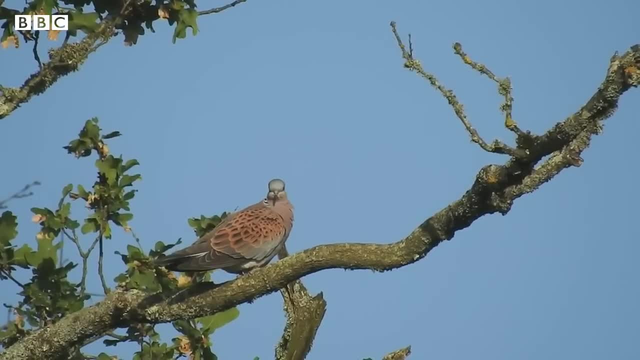 The UK is one of the most nature depleted countries in the world, with just half of its nature richness remaining. The Worldwide Fund for Nature. the Worldwide Fund for Nature is one of the most depleted countries in the world, with just half of its nature richness remaining. 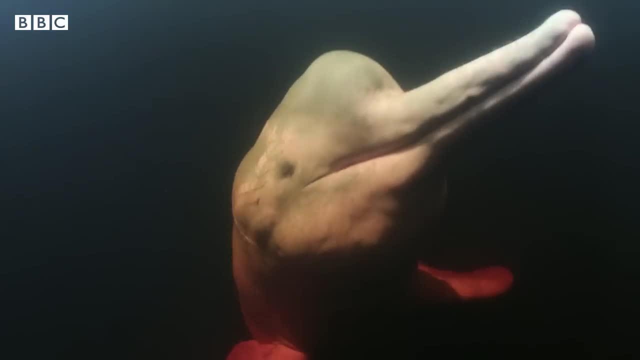 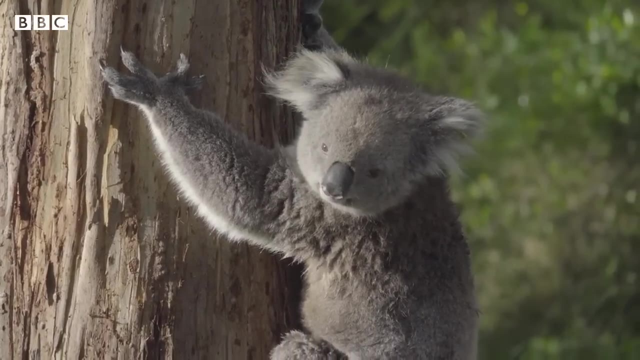 The Worldwide Fund for Nature. the Worldwide Fund for Nature says it's now or never if we're to restore the natural world. The government says it's committed to halting the decline of nature by 2030 and that it will continue to improve on wildlife laws. 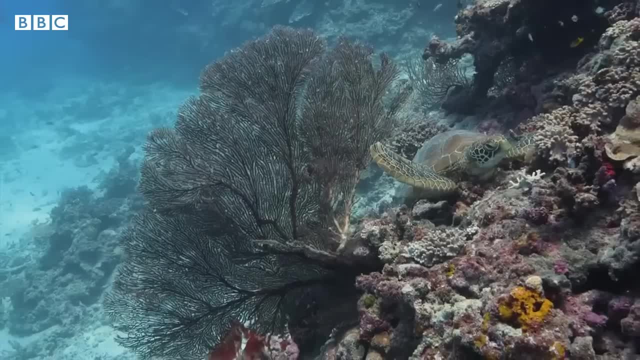 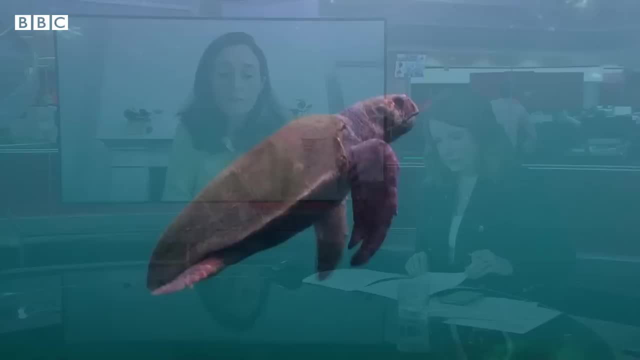 But the WWF says it needs to act very quickly if it wants to protect species from danger and distinction. Sean Dilley, BBC News And we can get more now on that from the WWF, which has just released that report. They're UK chief executive. 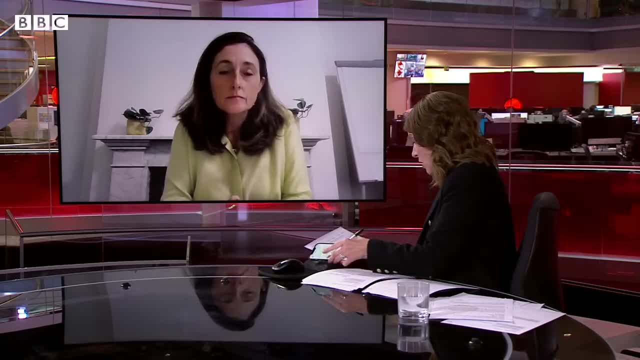 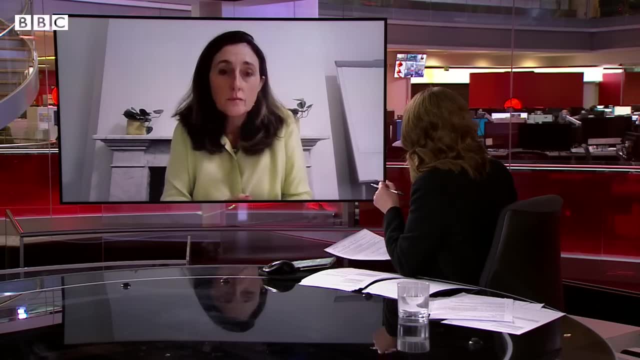 Tanya Steele joins me now. Tanya, thank you very much for your time. That is a lot of loss in a very short time: Nearly 70% decline in just under 50 years. Put that in further context for us, Tanya. 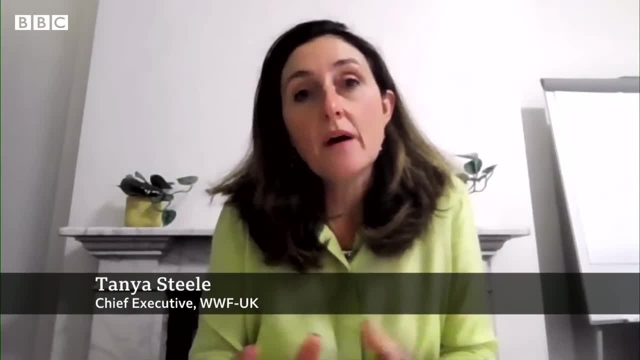 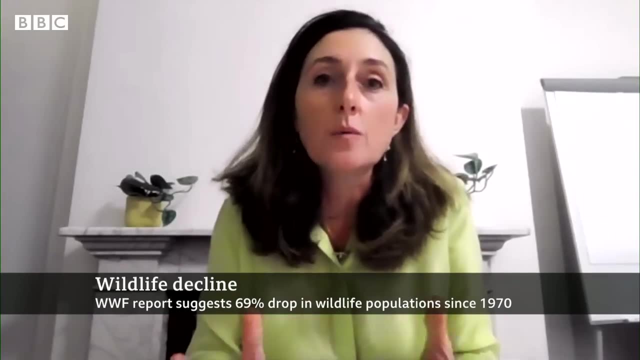 I mean, this is our most comprehensive report ever And it is a stark warning for us. If wildlife and its habitats don't survive, then neither will we. And if we were to treat the human population as one species that we were monitoring, 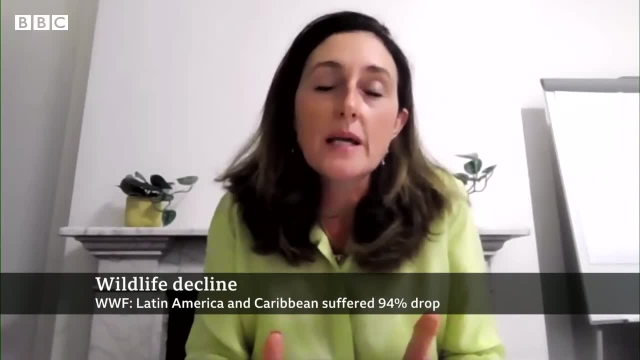 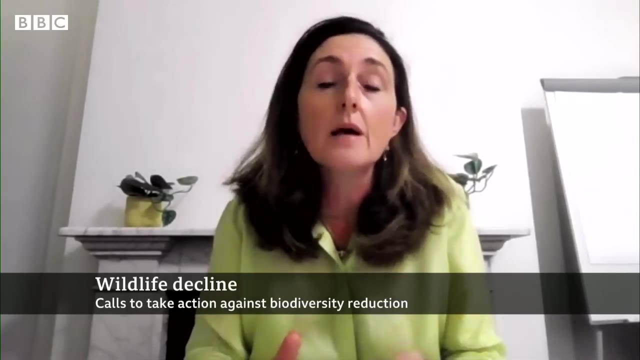 it would be the equivalent of wiping out the entire populations of China, Europe, Oceania, the Americas combined. So this is a devastating set of impacts for our natural world, And probably what is even more devastating is that we have reported these declines repeatedly. 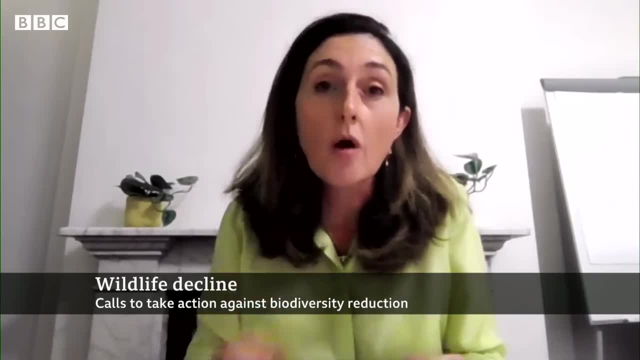 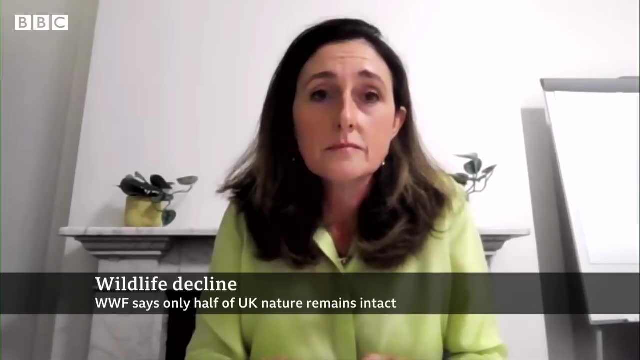 but we have seen very little action from world leaders to start to halt this loss and to put it onto a path for recovery, And in fact, you were telling me about this And we spoke at COP26 in Glasgow last year, Tanya. 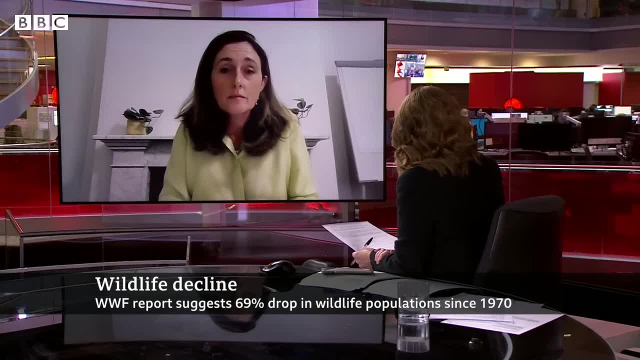 Since then, have you seen any plans, any initiatives from governments anywhere around the world that give you hope that someone's actually taking this seriously, really doing something about it? I mean, I think that for the most part, many world leaders have been missing in action. 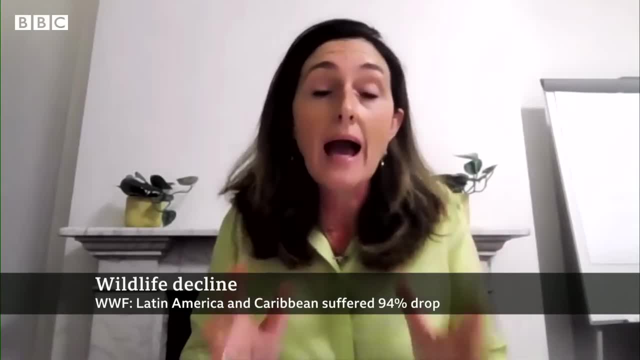 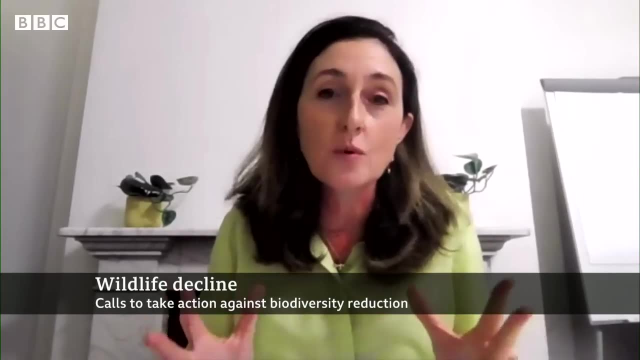 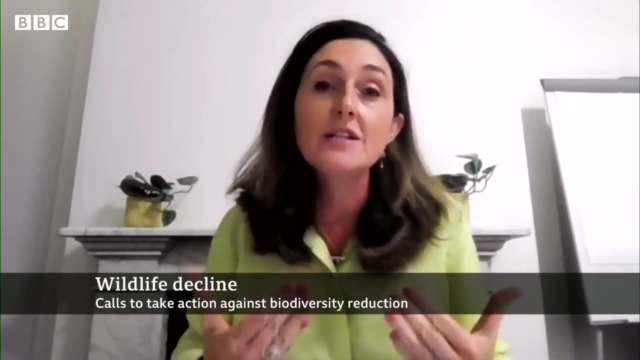 And we really do need those leaders to act and galvanise now, Because nature is the linchpin in the fight against climate change And the loss of our natural world is shocking enough, But we have the greater peril of climate change really kind of heading to us at high speed. 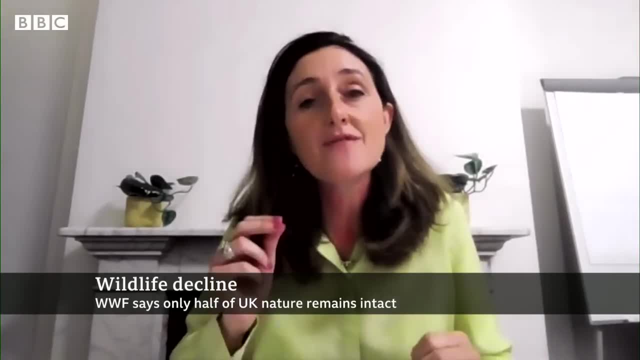 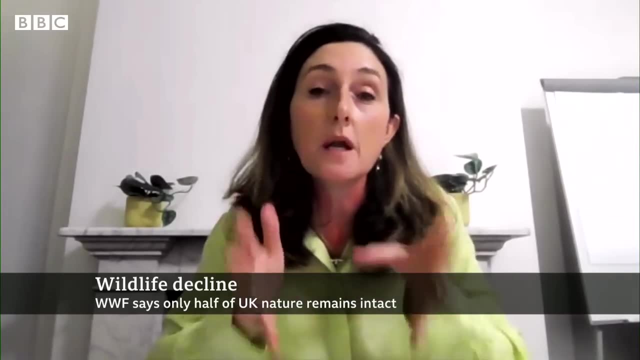 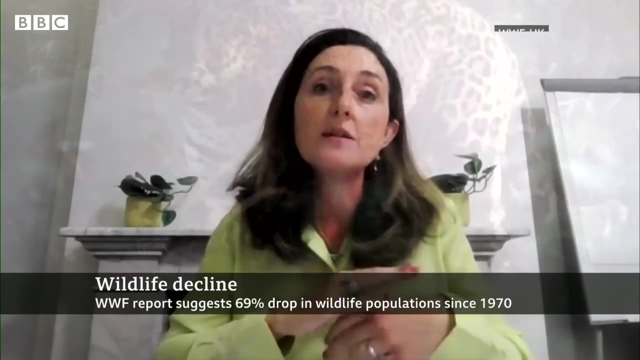 So to not address the loss in our natural world means we have no hope at all of reaching one and a half degree targets. And we have a very short window of opportunity. There is a global leaders meeting in Montreal in December where a new action plan needs to be formed to really start to halt this loss of nature. 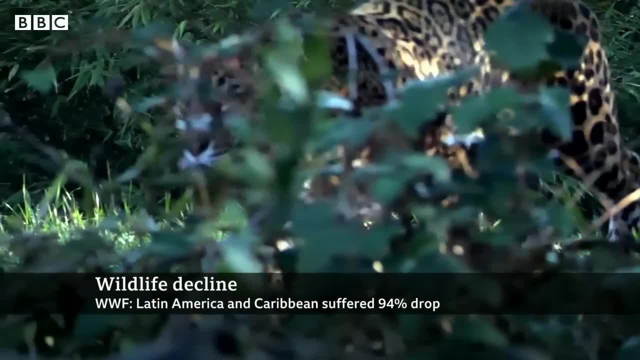 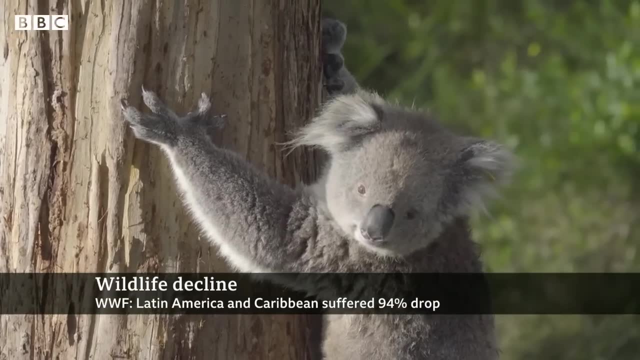 and actually start to regain control of the environment, And we need to recover it, And anything less, anything less than an agreement to do that would be an utter betrayal of future generations. I'm just trying to understand why it isn't being taken seriously enough. 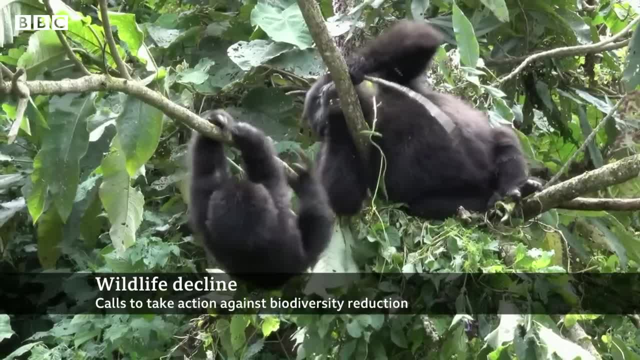 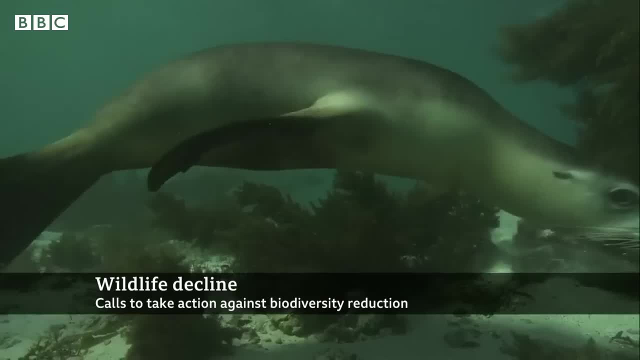 I mean, yes, the words are all there, aren't they? People say we must do more to support our wildlife, our environment, But why is the time, the resources, the money, the energy not being put into the sort of plans? 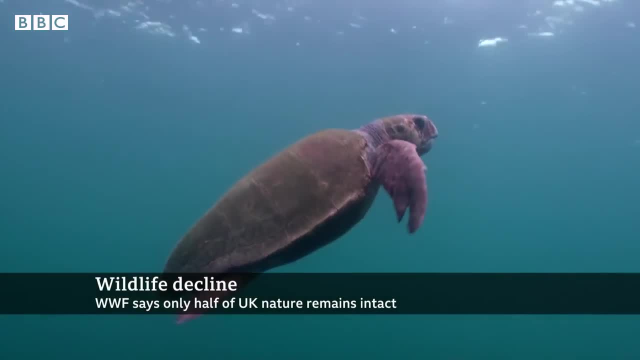 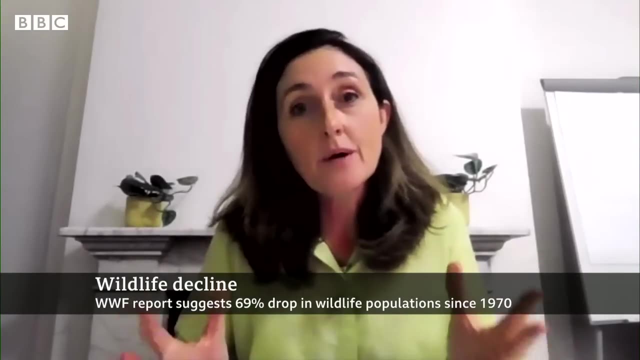 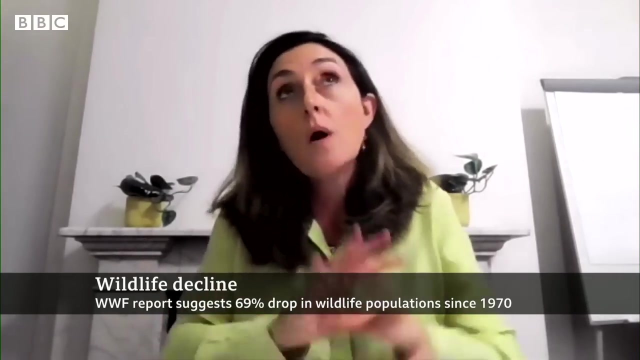 that you want to see to help protect animals. I think really it's taking time to get this issue up the political agenda. But I mean just the summer we've had. we've all experienced across the world here in the UK with soaring temperatures of 40 degrees, wildlife, wildfires across the whole of Europe. 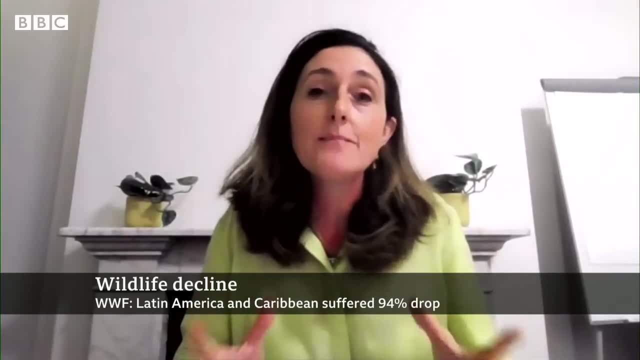 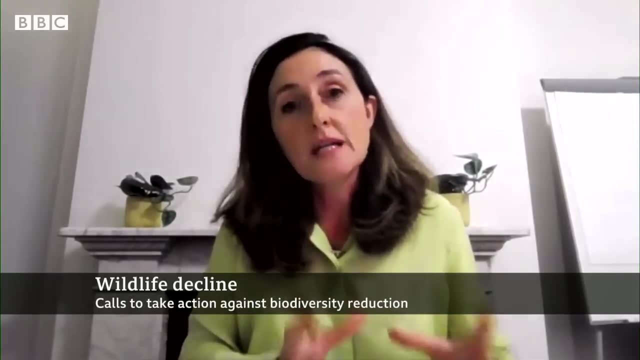 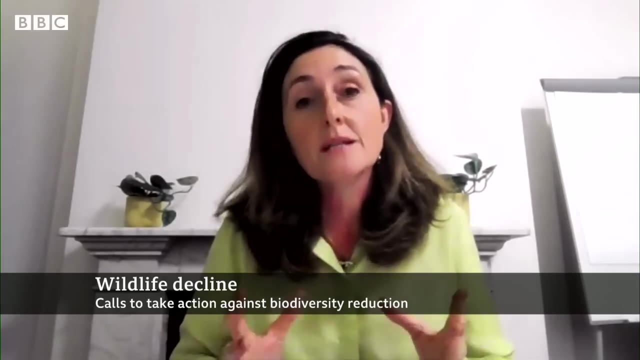 and biblical-style floods. level floods in Pakistan are starting to bring this to the fore And I think, realistically, we know that this is not just an issue that affects the ecology of our world. It is affecting our economies and it is affecting our ability to function as a society. 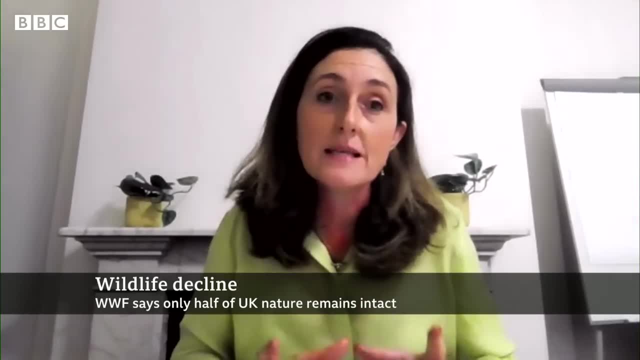 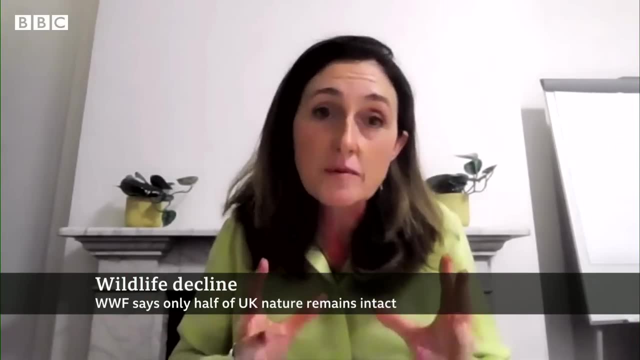 So we see this as an opportunity for world leaders to recognize that that we cannot continue to kick the can down the road And we have to actually focus on efforts beyond conservation, which are important, but actually start to reach into our supply chains, our economies and really how we work, because 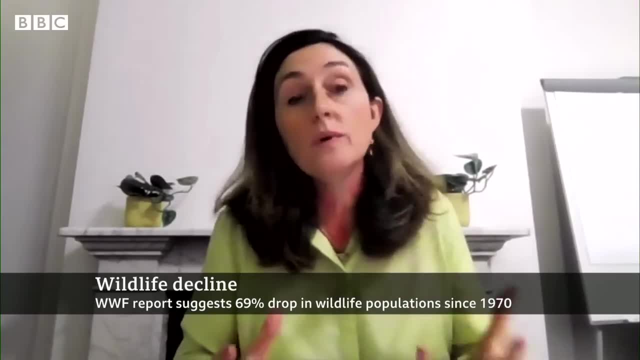 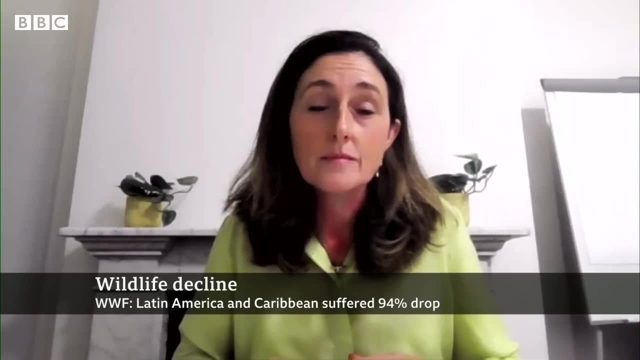 we are destroying so much nature by the way we live and work and consume as human beings, And it is no longer sustainable. Tanya, thank you very much for your time today. Tanya Steele, the WWF's UK Chief Executive.